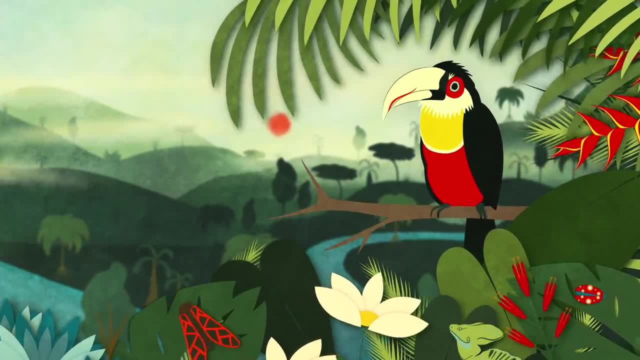 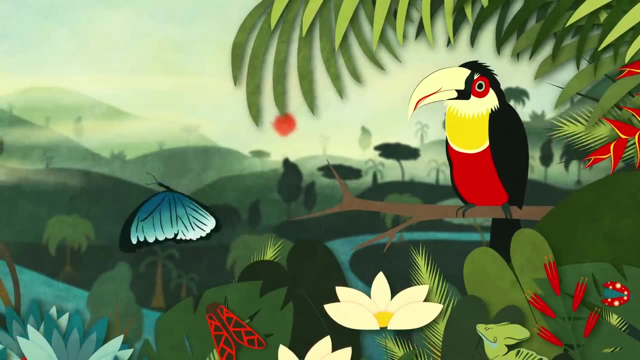 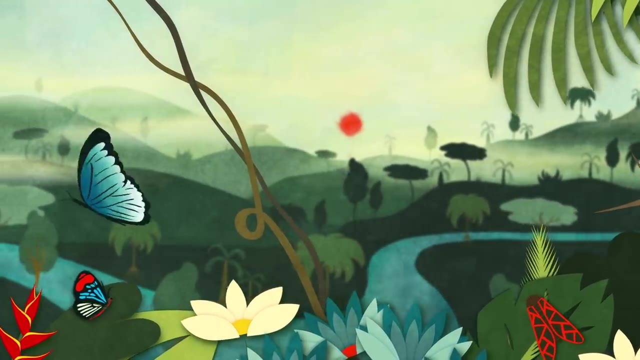 That weave is further reinforced by the genetic diversity within individual species, which allows them to cope with changes. Species that lack genetic diversity due to isolation or low population numbers are much more vulnerable to fluctuations caused by climate change, disease or habitat fragmentation, Whenever a species disappears because of its weakened gene pool. 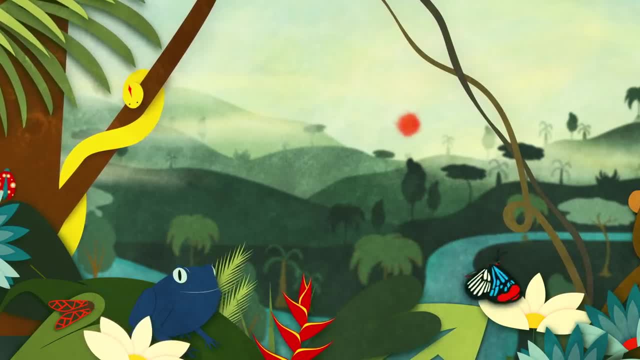 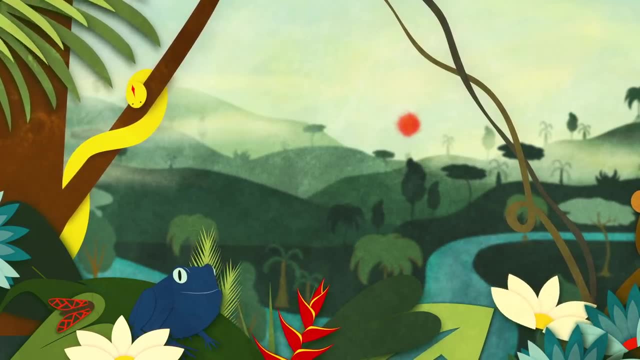 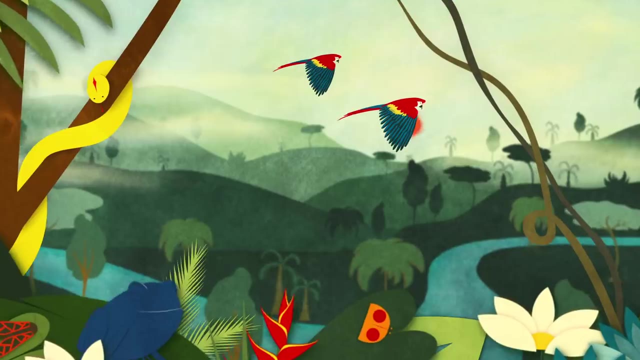 a knot is untied and parts of the net disintegrate. So what if we were to remove one species from the rainforest? Would the system fall apart? Probably not. The volume of species, their genetic diversity and the complexity of the ecosystems form such rich biodiversity. 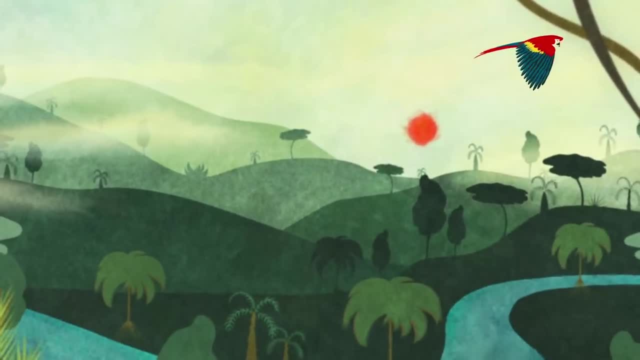 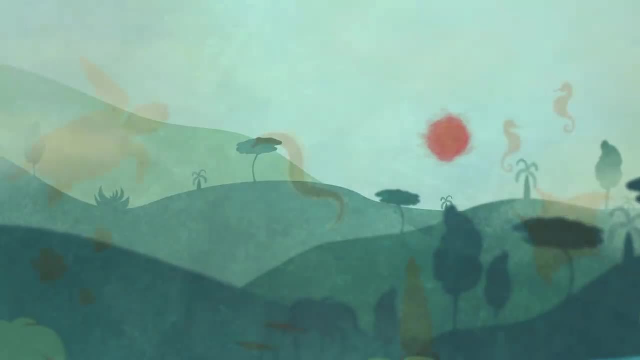 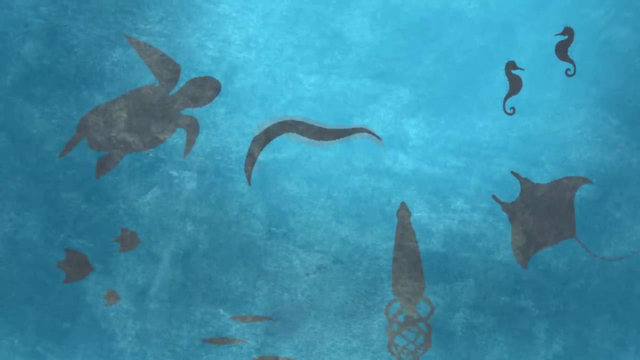 in this forest that one species gap in the weave won't cause it to unravel. The forest can stay resilient and recover from change, But that's not true in every case. In some environments, taking away just one important component can undermine the entire system. 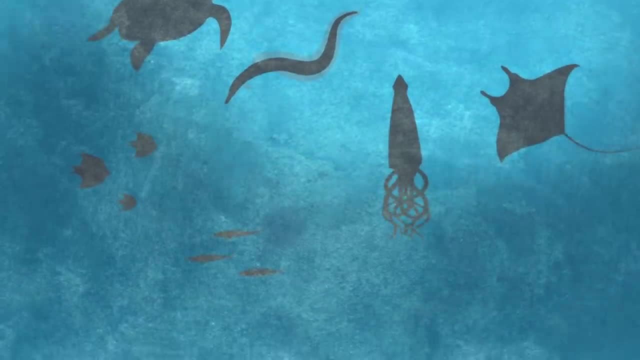 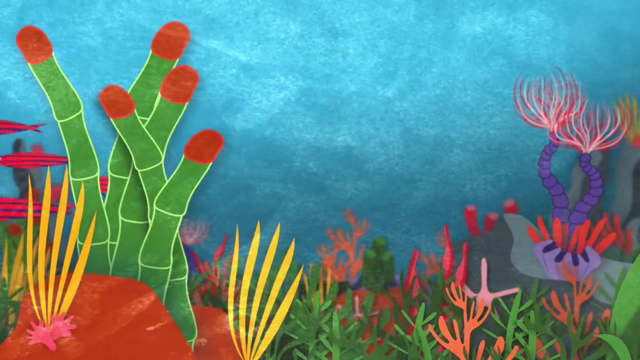 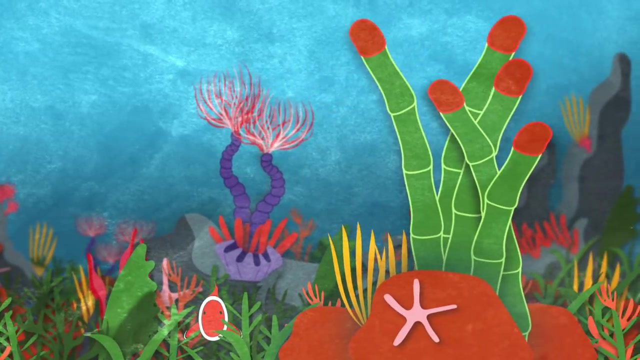 Take coral reefs, for instance. Many organisms in a reef are dependent on the coral. It provides key micro-habitats, shelter and breeding grounds for thousands of species of fish, crustaceans and mollusks. Corals also form interdependent relationships with fungi and bacteria. 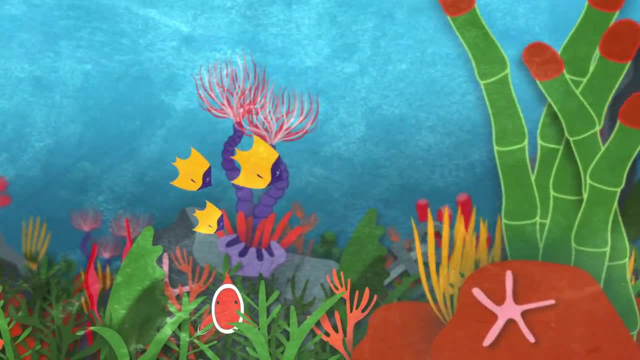 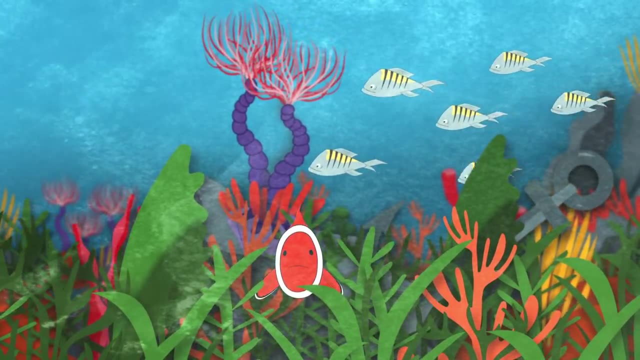 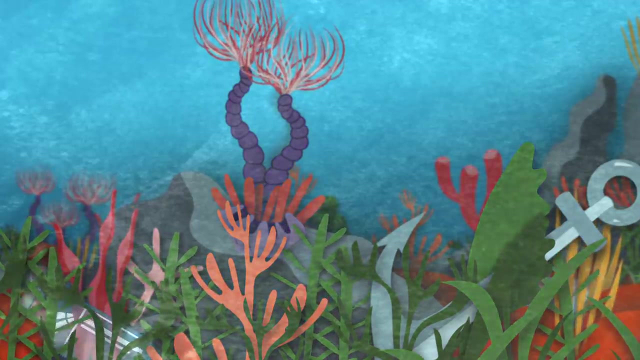 The coral itself is a loom that allows the tangled net of biodiversity to be woven. That makes coral a keystone organism, one that many others depend on for their survival. So what happens when destructive fishing practices, pollution and ocean acidification weaken coral? or even kill it altogether. Exactly what you might think, The loss of this keystone species leaves its dependents at a loss too, threatening the entire fabric of the reef. Ecosystem, species and genetic diversity together form the complex, tangled weave of biodiversity. 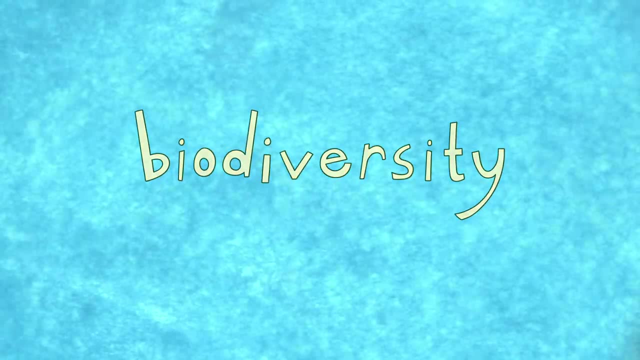 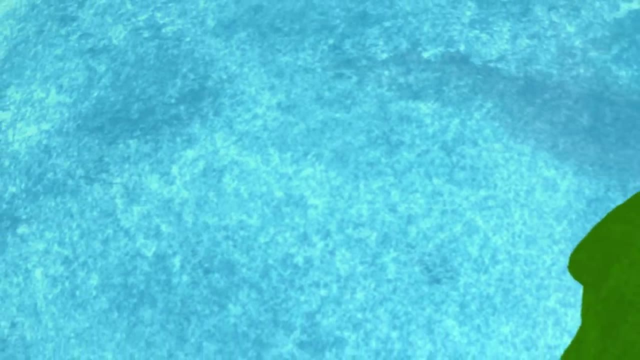 that is vital for the survival of organisms on Earth. We humans are woven into this biodiversity too. When just a few strands are lost, our own well-being is threatened. Cut too many links and we risk unraveling it all. What the future brings is unpredictable. 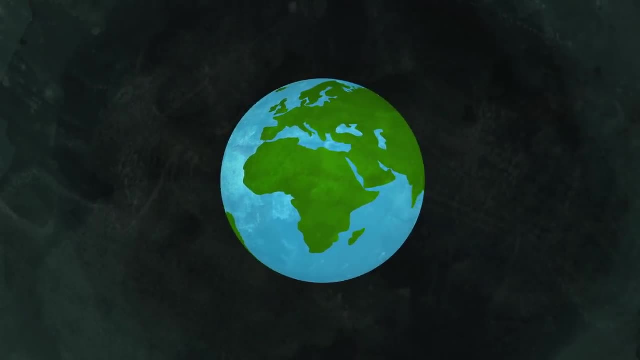 but biodiversity can give us an insurance policy, Earth's own safety net to safeguard our survival.